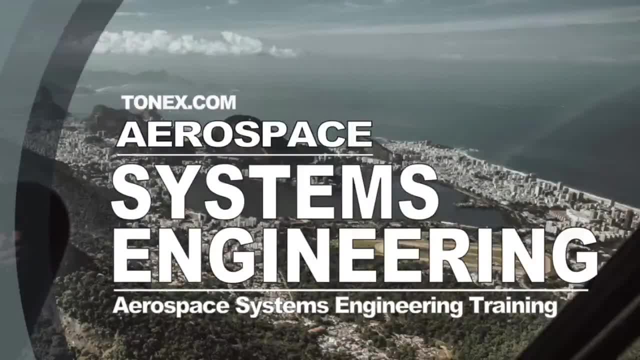 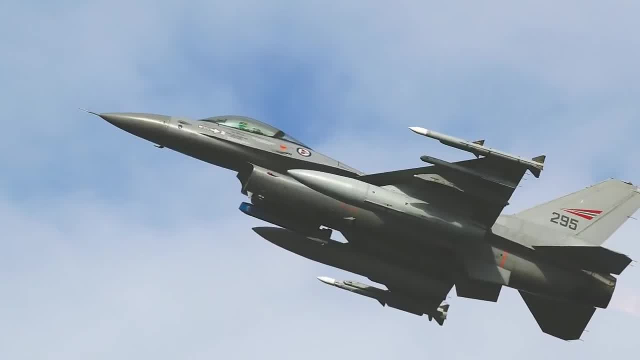 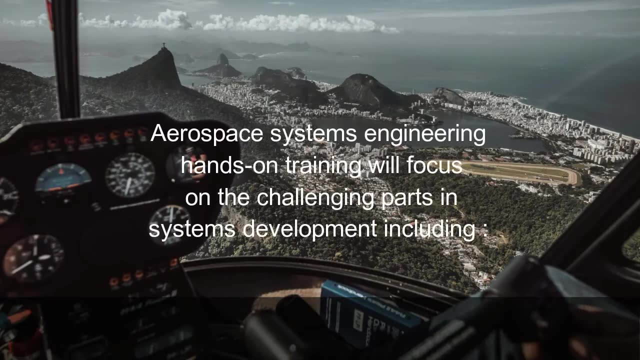 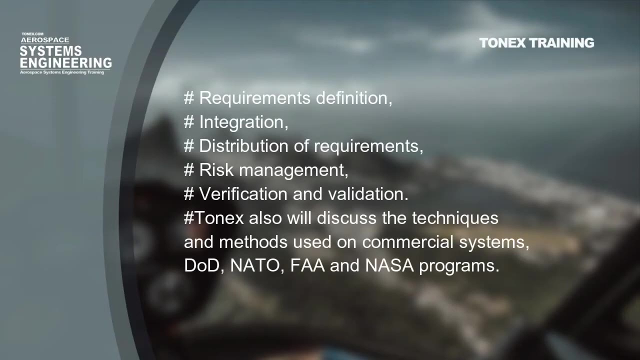 Aerospace systems engineering hands-on training will focus on the challenging parts in systems development, including requirements definition, integration, distribution of requirements, risk management, verification and validation. tonex also will discuss the techniques and methods used on commercial systems, DOD, NATO, FAA and NASA programs. aerospace systems engineering training. 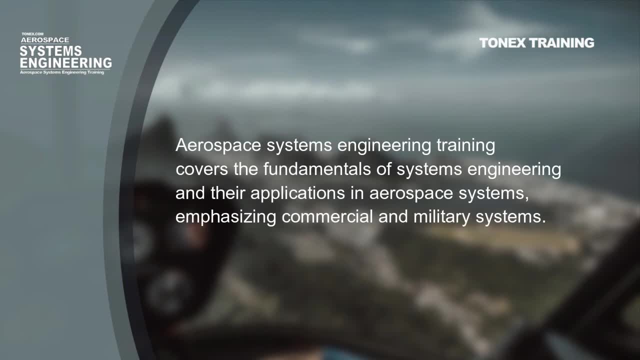 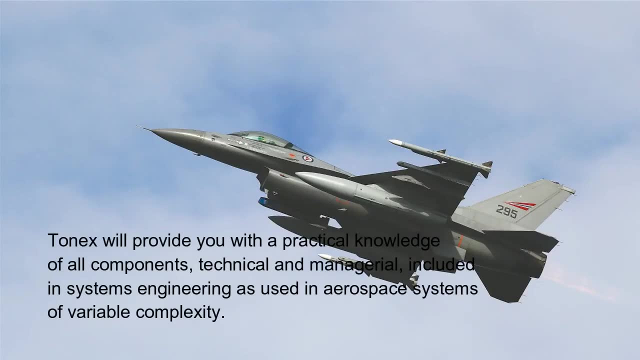 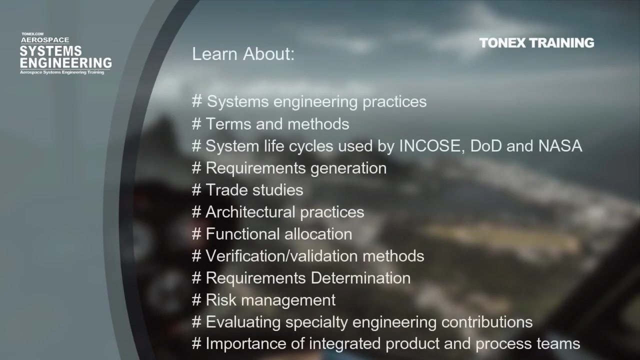 covers the fundamentals of systems engineering and their applications in aerospace systems, emphasizing commercial and military systems. tonex will provide you with a practical knowledge of all components- technical and managerial- included in systems engineering as used in aerospace systems of variable complexity. learn about systems engineering practices, terms and 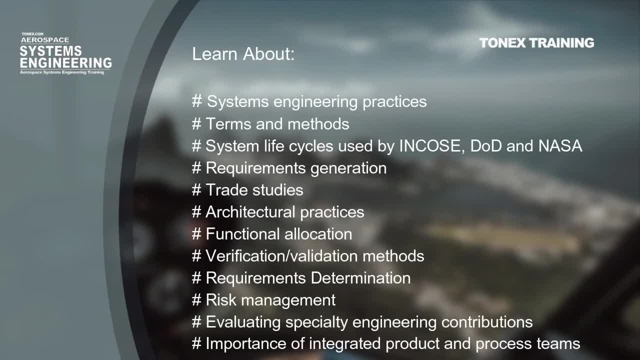 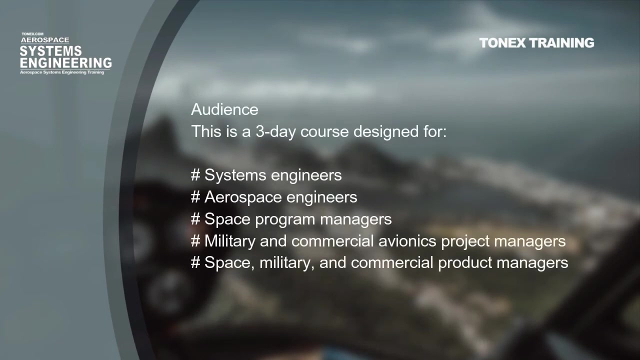 methods, system life cycles used by in goes, DOD and NASA: requirements generation, trade studies, architectural practices, functional allocation, verification, validation methods, requirements determination, risk management, evaluating specialty engineering contributions, importance of integrated product and process teams. audience: this is a three-day course designed for systems engineers, aerospace engineers, space program managers, military and commercial avionics project managers, space. 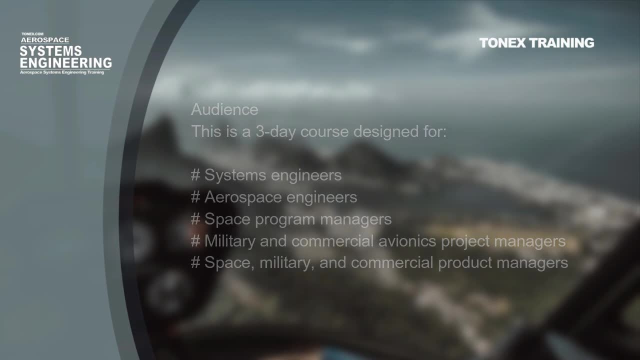 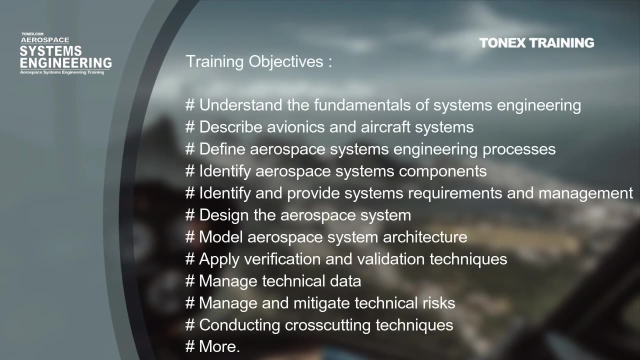 military and commercial product managers. training objectives: understand the fundamentals of systems engineering applied to aerospace industry. describe avionics and aircraft systems. define aerospace systems engineering processes. identify aerospace systems components. identify and provide systems requirements and management. design the aerospace system model aerospace system architecture. apply verification and validation techniques. manage technical data. manage and mitigate technical